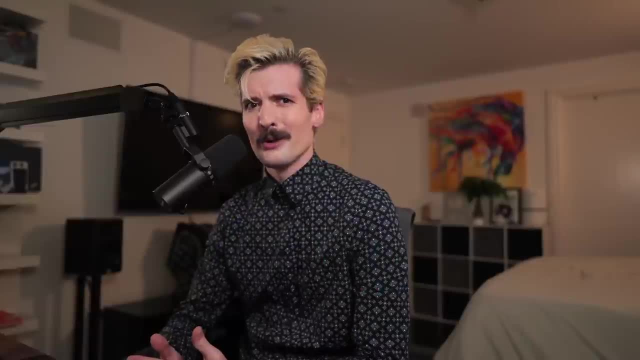 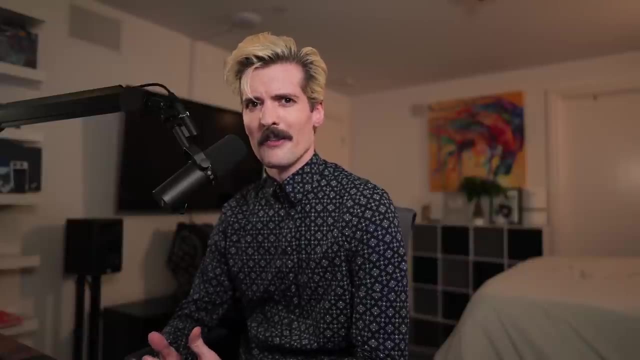 today, Things like Twitter, YouTube and so many more built with these awesome libraries to make surprisingly good applications And, as such, most developers who build user experiences on the web are building with component libraries, which is why I'm here to tell you that they're dying. 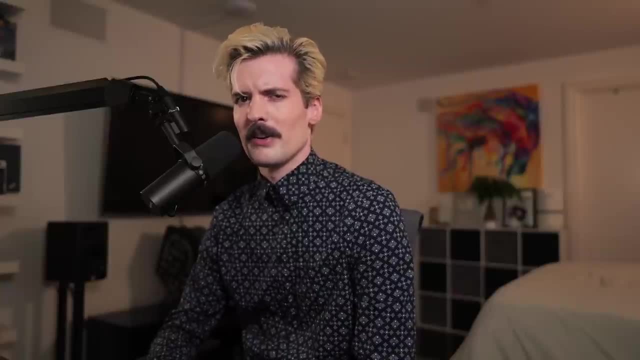 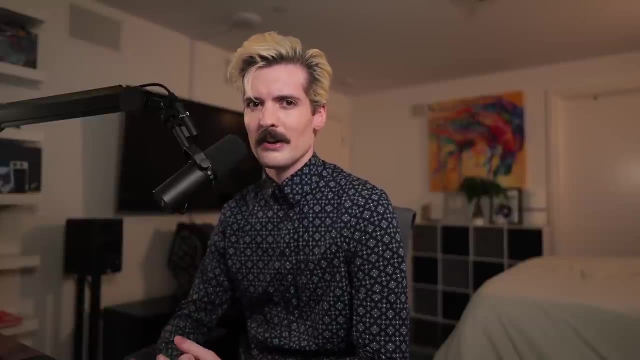 The future is not one of big popular UI libraries that everybody is NPM installing and building within their codebases. It actually looks quite a bit different. I've been thinking a lot about this and I wanted to share my conclusions. after thinking about it for too long and where I think, 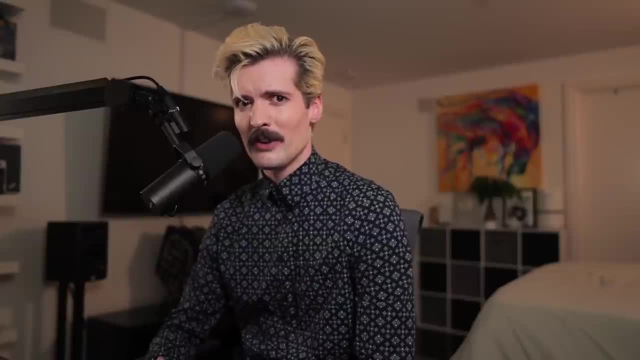 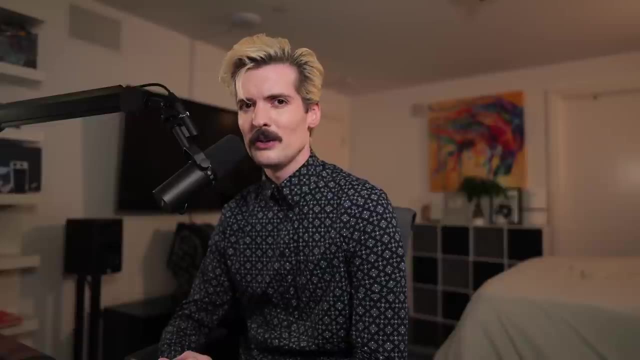 things are going in the future of the web. I want to be clear: this is a very speculative video based on trends I have been seeing and experiences that I've been impressed with as things change over time. But I really do see a trend happening here and I wanted to take the time to document it. 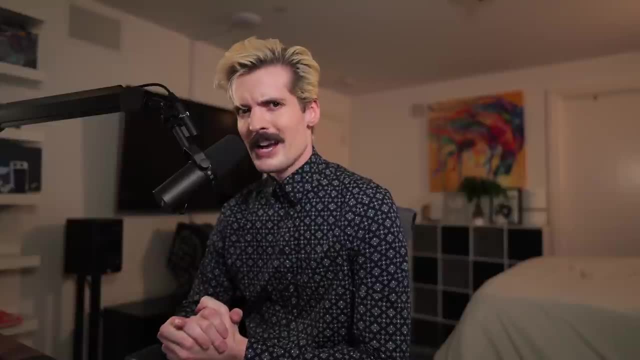 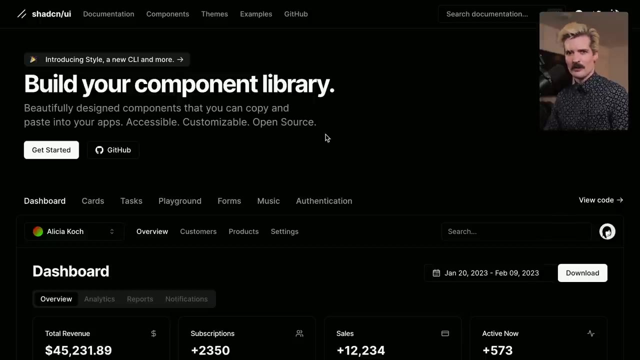 and share my thoughts. So let's talk about ShadCN and ShadUI. If you're not already familiar with ShadCN UI, it's an awesome open-source project by ShadCN, a prolific open-source contributor. in recent addition to the team at Vercel. He helped a lot with vZero and a lot of the other cool stuff going. 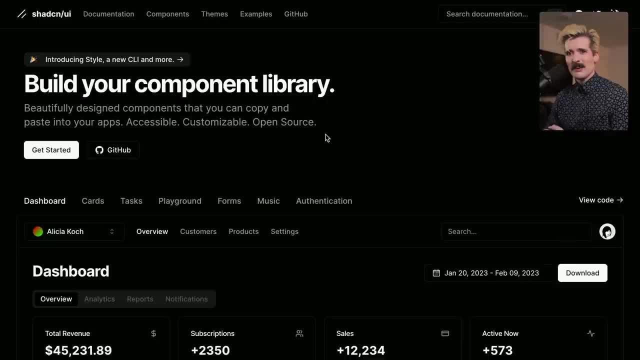 on there. But what is ShadCN UI? Isn't this a UI library? Well, kind of not really. It's the pieces for you to build the perfect UI library for yourself. As it says here: build your component library. What ShadUI provides isn't a package that you can build yourself. It's a package that you 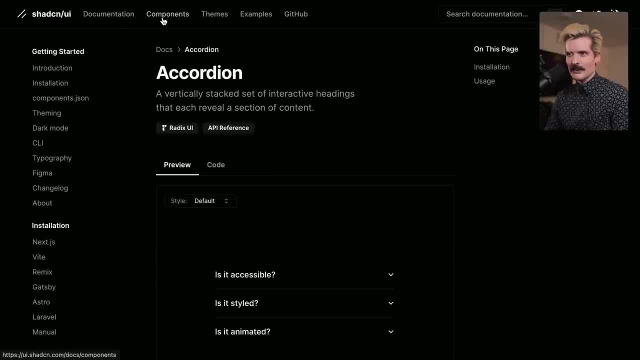 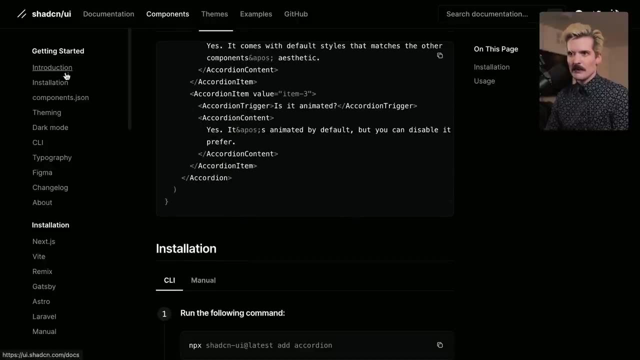 install. They do have a CLI to help you set things up, But the way ShadCN works is it installs things in your code base as actual code you can edit When you set up any of the elements in here. you can either manually grab the files that you need and copy paste them into your app. 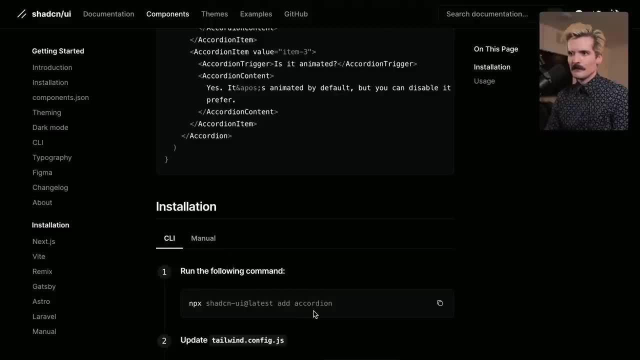 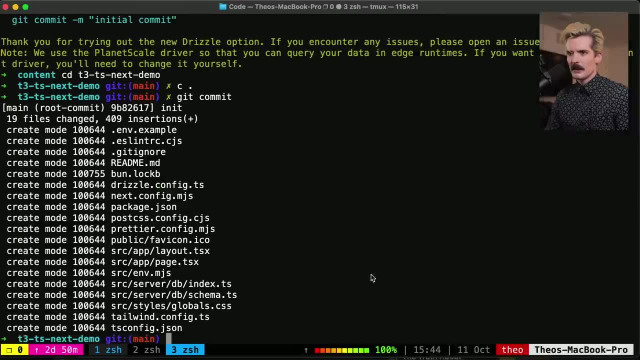 set up the Tailwind, set up all these things. or, as of recently, you can run this command. So let's go add the ShadCN accordion. Oh, look at that, They have options for all these different runtimes. I just copied the bun command. fourth times the charm. 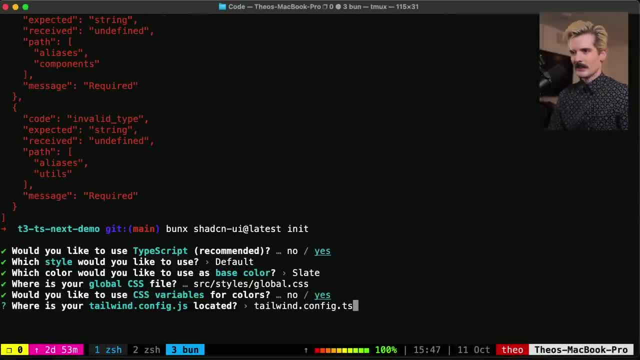 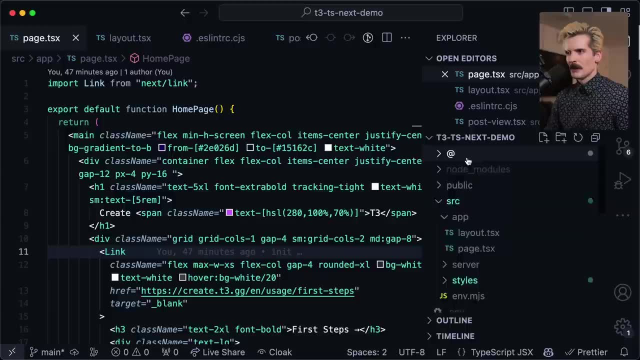 Tailwind, tailwind, Tailwind, tailwind, Tailwind, tailwind. dot config, dot ts. i wish it was smart enough to auto detect this stuff. i didn't want to change the alias, i want to change where these actually go. but that's fine if it's putting it in this. 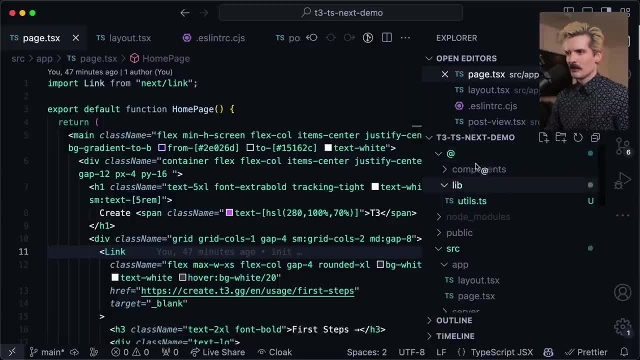 at slash thing. i don't want to fuck with it too much. yeah, it should work, but it'll be a pain to manage later. move it now, i will trust you. cool, we'll move this where i want it because, again, like, the magic of this is that it's actual code i own. i think they are smart enough to update. 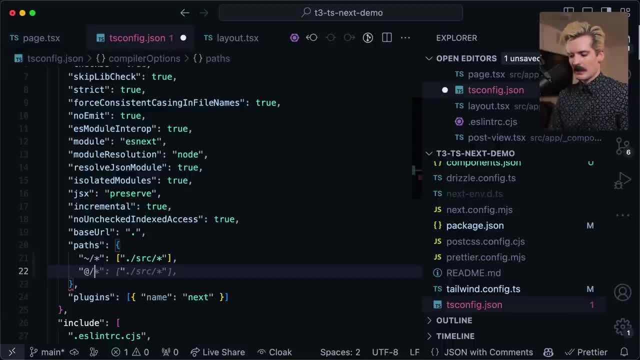 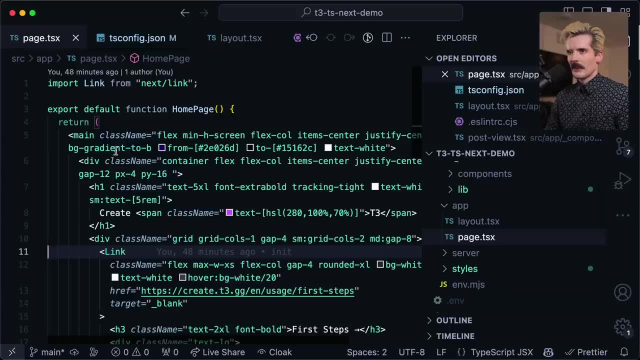 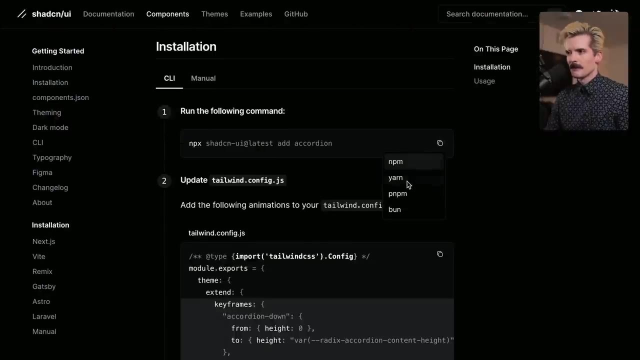 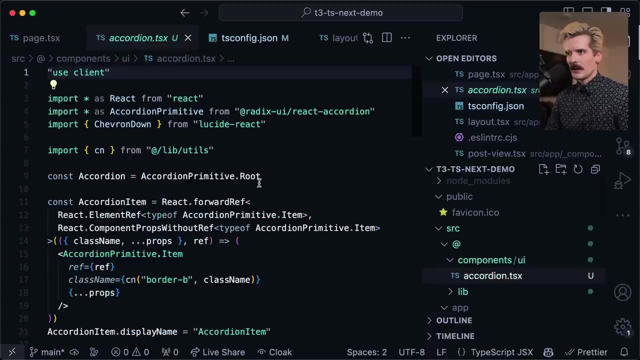 this. they're not, so i'll add at slash star to be dot slash, source: slash at slash. cool. so now i've done that, i should be able to install components. so if i want that accordion thing, scroll down here. yoink, and now i have in my own code an accordiontsx file and if i want to make any changes, 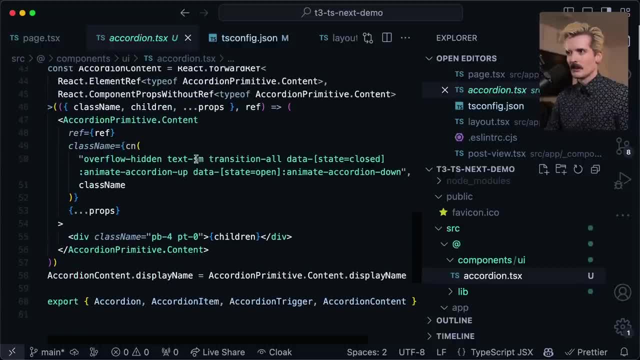 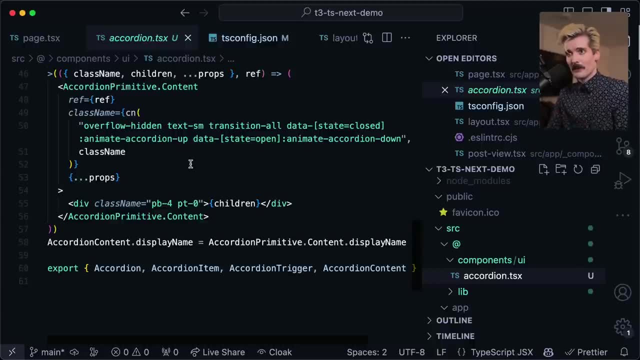 to this i can, because it's my code and my code base, using tailwind, the way i personally would like to use it. it's also built on top of radix ui, which makes it way easier to have accessible components and all the components in shad ui. 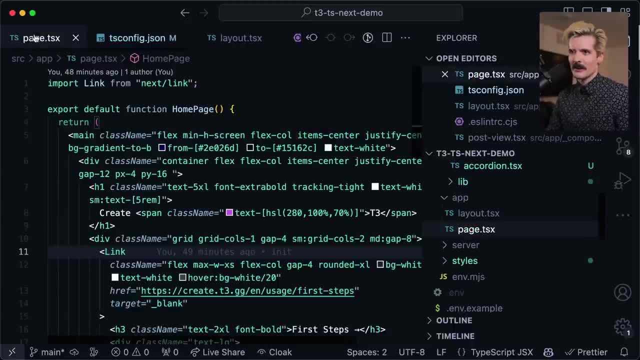 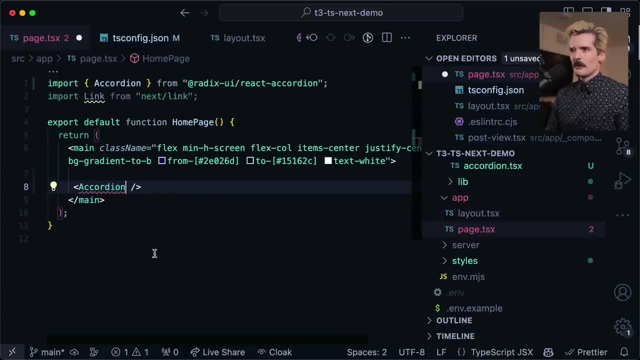 are incredibly accessible. there's a lot of contributors making sure it stays that way, so if i wanted to go in here and just delete a bunch of this code, i hate how scroll works in vs code sometimes when you're selecting things: import accordion not from react accordion at slash. 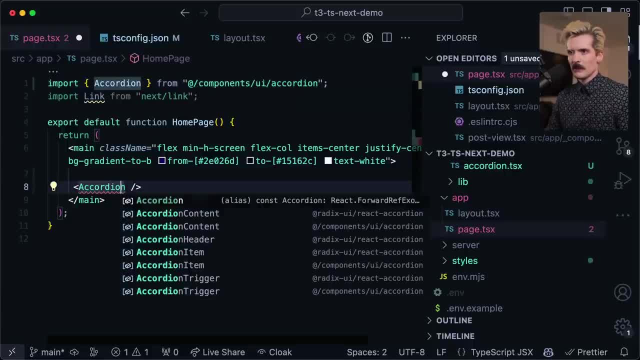 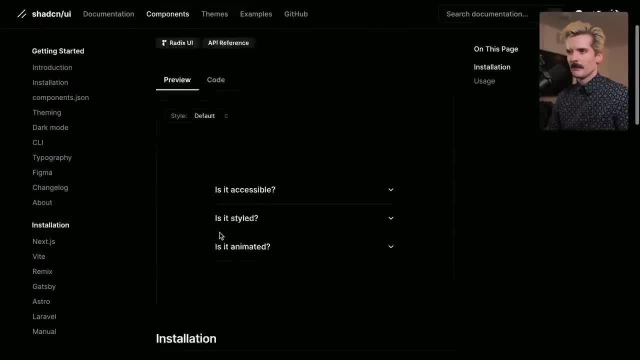 components: ui accordion. it's going to need some props, i'm sure. what does it want? type equals single- cool. we can also look at how they actually use it in here. there's a code example: accordion type single- collapsible. it has accordion items in it. let's just grab this first item. 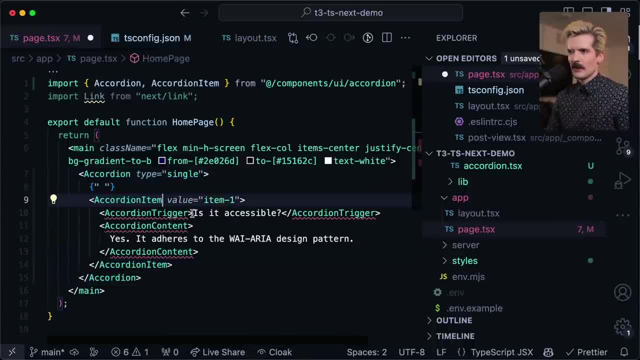 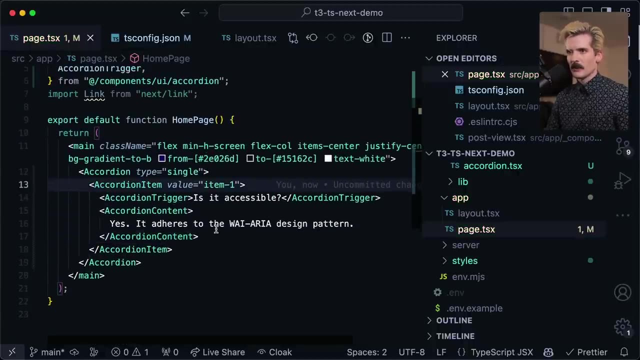 obviously a lot of these need to be imported. a little annoying that it's confusing the radix ui imports with the shad cn ones. i almost wish there was a way to tell typescript to never use the radix ui ones. but now we have what should be a totally functioning, nice looking accordion. 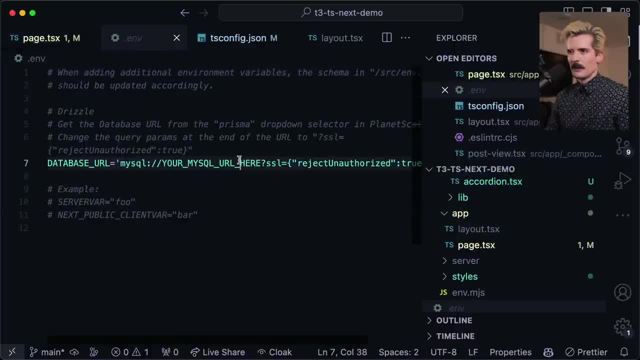 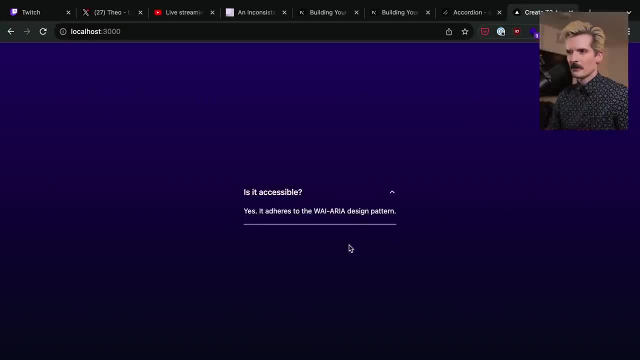 oh, it's not going to work, so i don't have environment variables. i'll just go make a nonsense one. there we go. now we have a fully functioning collapsible accordion and our code that behaves the way we want it to, and i know that was a bit of work to set up, but it wasn't. 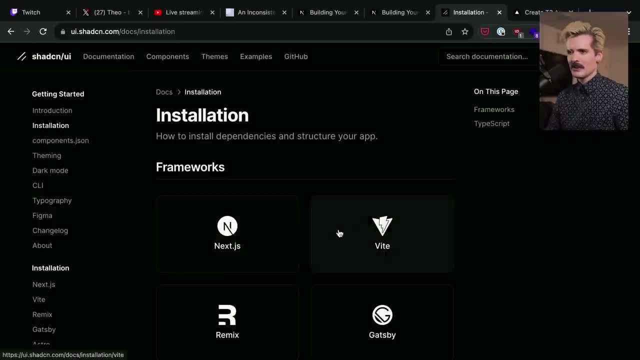 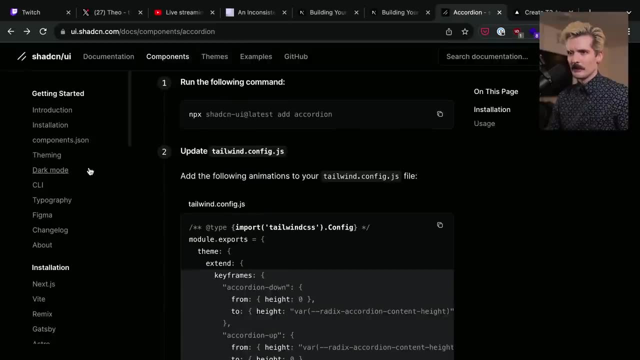 that bad and it's mostly because of where i'm putting things. and again, the cli that they just added is very new and we'll smooth out those parts. but now, if i ever want to add new elements- it's trivial too- i can scroll and find collapsible. 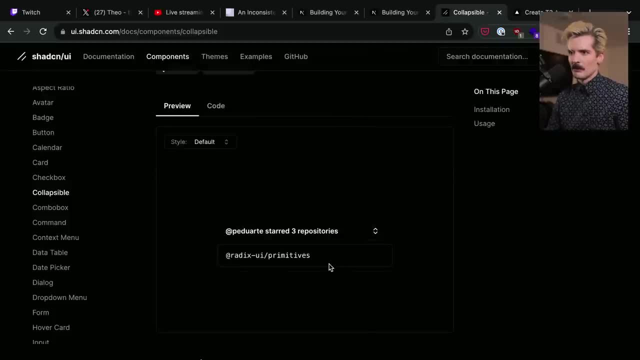 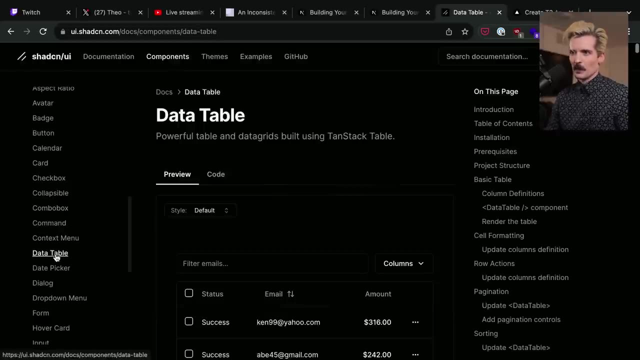 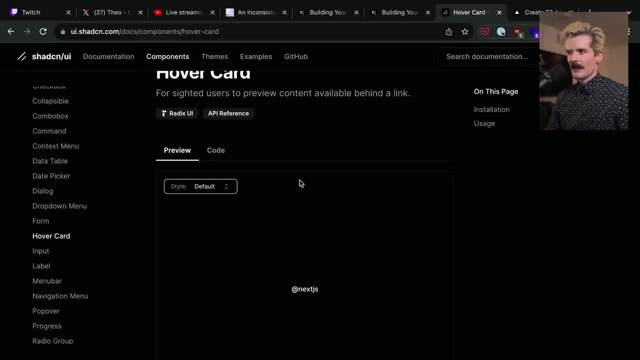 here's a collapsible repo selector. who hasn't had to build one of these before? or a combo box where you select multiple things at the same time, with a search built into, or a data table or a hover card. all these types of things are very annoying to build and now we have. 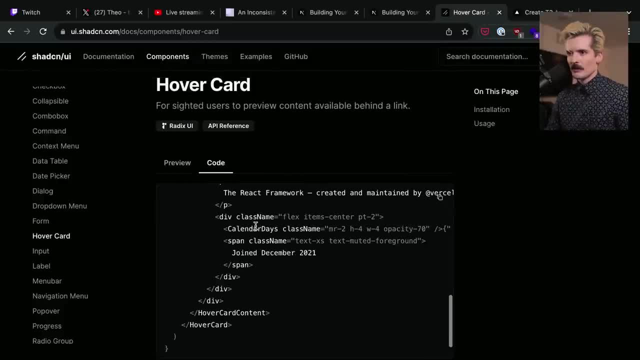 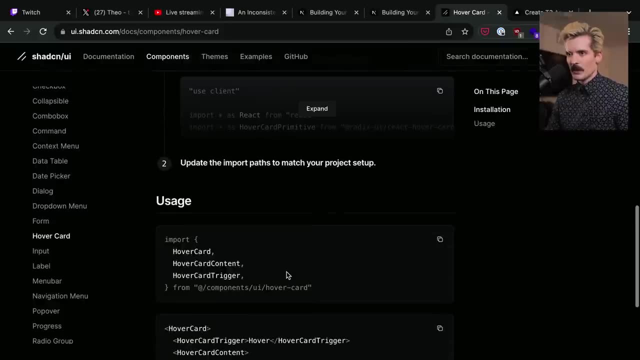 code we can rip immediately. you can always grab the code directly. it's one of the options when you set up. but you don't have to. you can use the cli or you can use the manual copy paste thing of parts, because all of this code is meant for you to run in your own code base. that's what's. 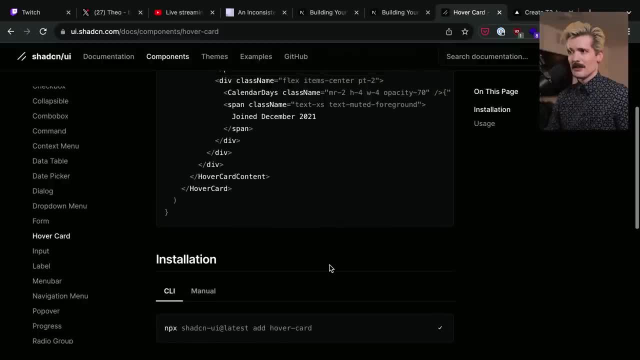 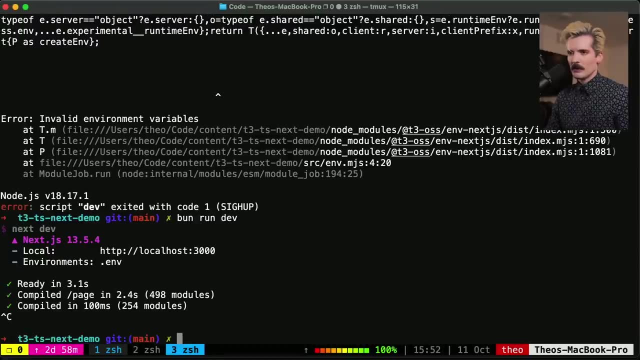 so different about this for me is i don't think about installing one specific package or one specific ui library and hope it has the solution, and if it doesn't, i'm screwed. it's very easy now to just run this command and add a hover card. now, if i go to my source, you'll see i have hover. 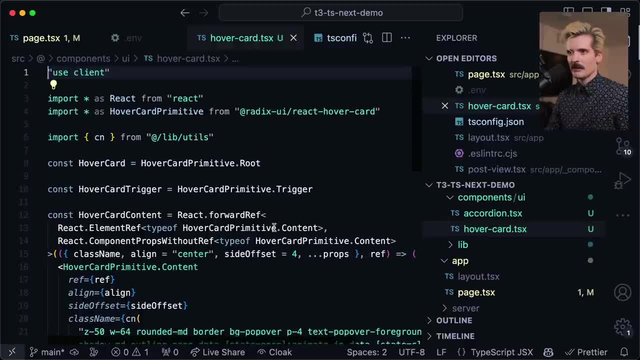 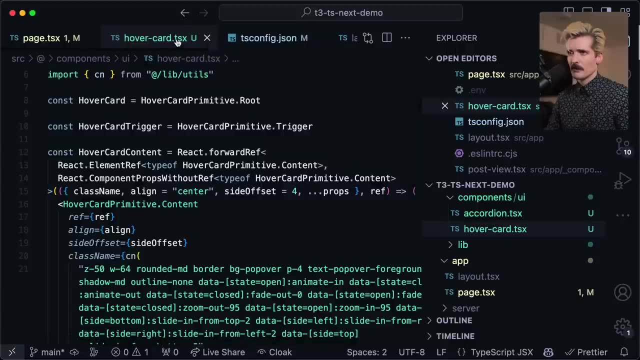 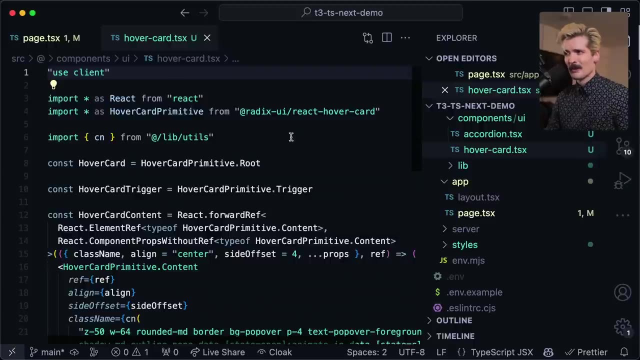 cardtsx, which is a complex component library file in my code base that i can change however i want. that's an incredibly powerful for developers of all types of ui stuff where a lot of the simplicity of a provided component library is there but, more importantly, the ownership you normally lose that exchange. 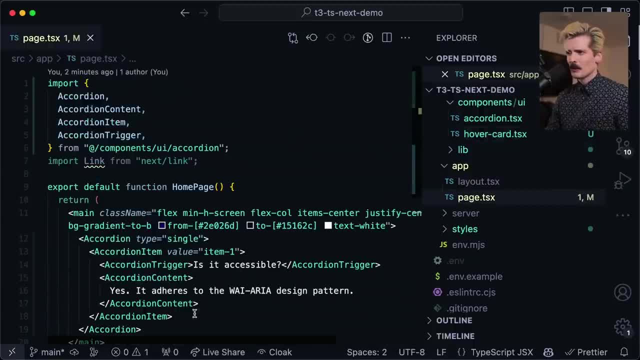 didn't happen. so if you're building a ui library for your company, this is one of the best starting points imaginable, and if you're just starting a side project and want a couple buttons or accordion like elements or all the different complex, accessible uis that many of us need to. 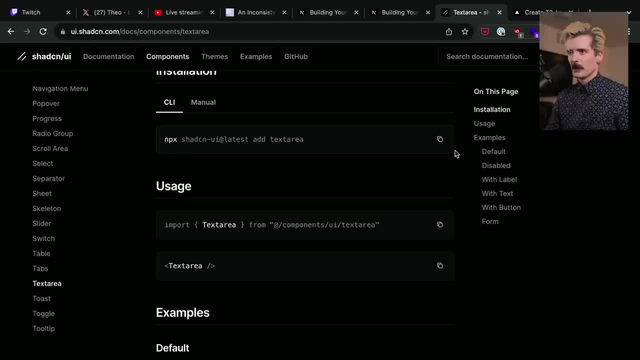 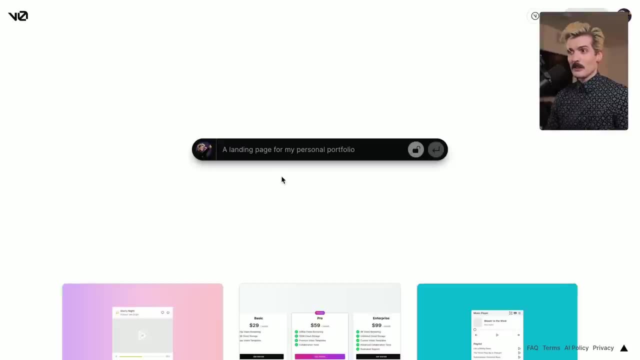 build all the time, just hopping in here, clicking the one you want, clicking the copy button and running this command lets you, in your code base, have whatever ui elements you need. where this gets much crazier is v0.dev, which, if you're not familiar, it's a new project by vercell that lets you generate 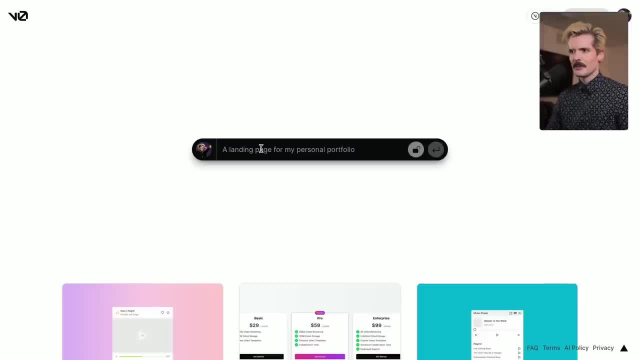 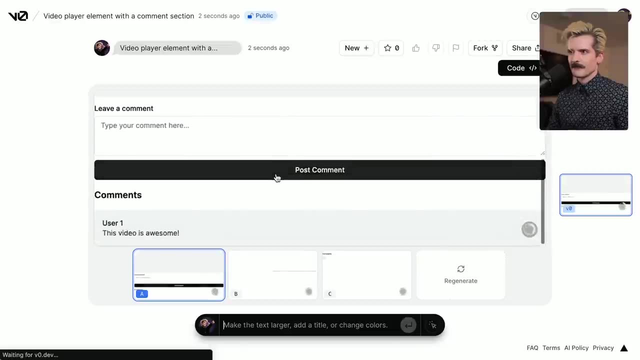 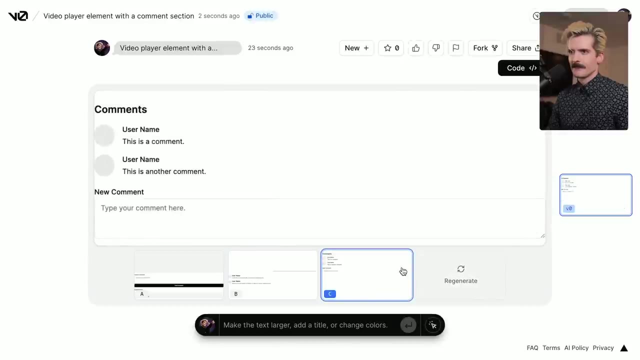 components built on top of shad cn with ai. so if i wanted to generate video player element with a comment section, now it's generating four different potential uis for a video player with a comment section. i didn't mean to hit regenerate. now it's going to. 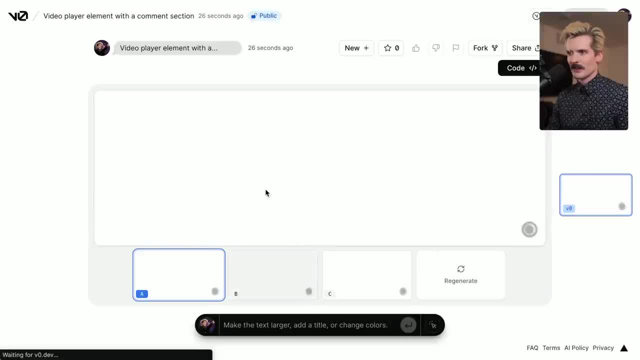 rerun all of that oops momentarily after it doesn't rerun because i accidentally hit the wrong button. i do kind of hate that regenerate is here next to all of these, because the ones i had before looked much better. this one looks fine. add your comment. 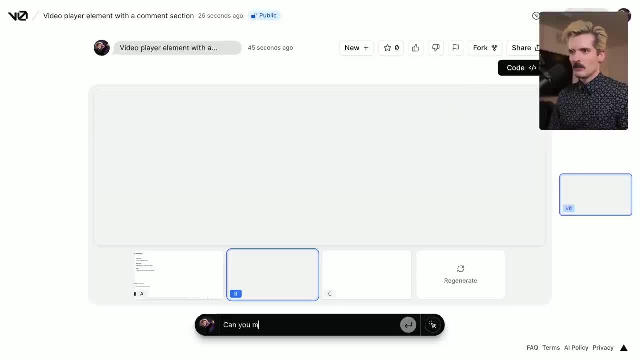 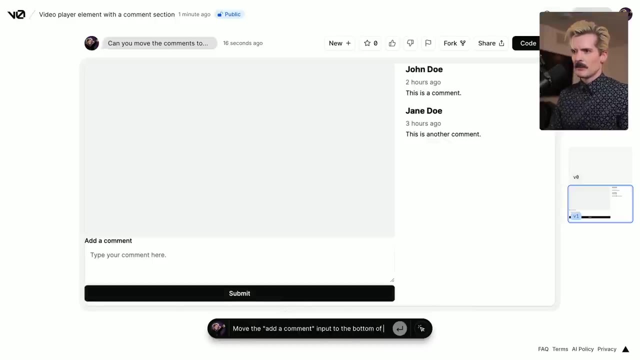 here's some comments underneath. let's ask it to make changes. can you move the comments to the right as a scrollable sidebar? move the add a comment input to the bottom of the comments sidebar at a title section below the video player. While this is generating, I'll take the time to point out that Vercel does sponsor the channel. 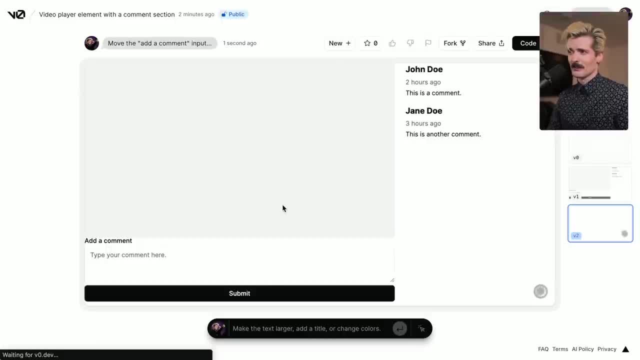 They have not told me to talk about V0 or any of this stuff. I just like it and genuinely use it and think it fits the theme of this video. So, no, they're not sponsoring this video, I'm just doing this because I wanted to. So yeah, And now one last request: Extend the comment section sidebar. 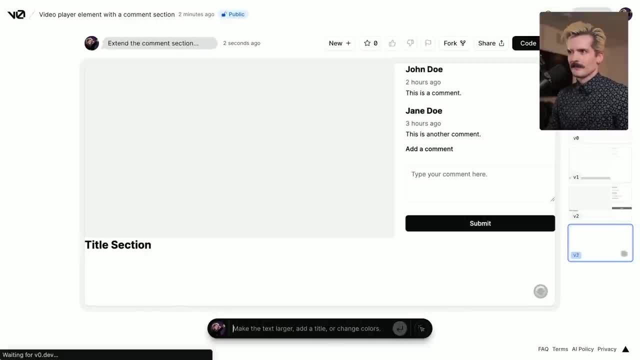 to be full height. And now through just a handful of requests to an AI generator. theoretically, once this runs, seems like we're getting a lot more traffic lately. Okay, I didn't like doing that part, But thankfully it is just generating code that we can rip into our code base. I click. 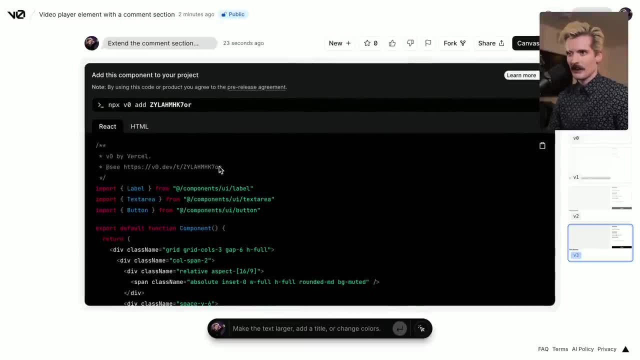 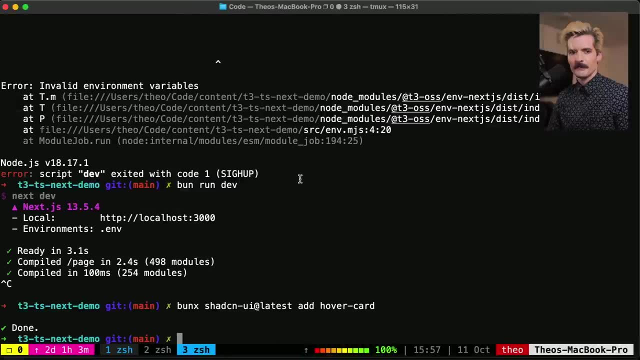 this little code button, we can see the exact React source it generated, as well as the HTML, if we wanted to just use the HTML in any other framework. More importantly though, I can copy the command, run this, name, the component and then run it again, And now I can see the. 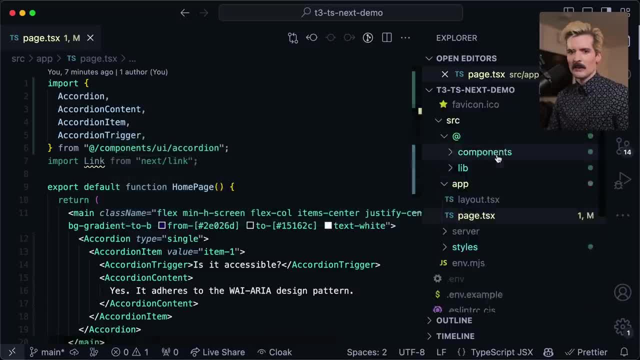 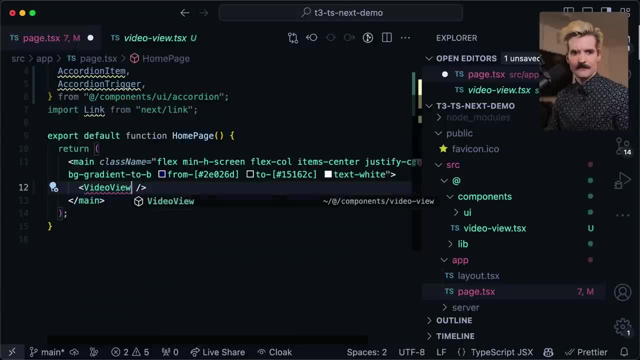 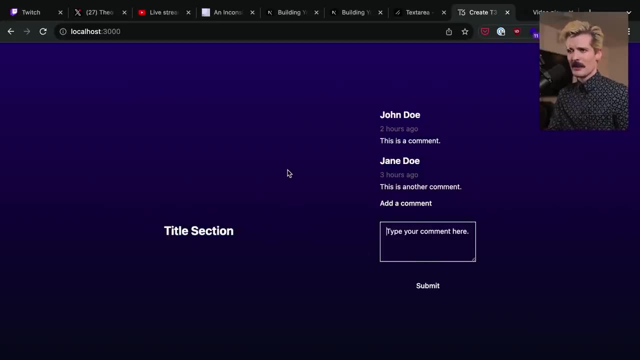 component: video view. And now, the same way we would add any other UI component, we have video view. dot TSX is a component I can mount, Just like that. And here is this basic component. Again, we have our own CSS on the page and that's going to affect things. We have a really good 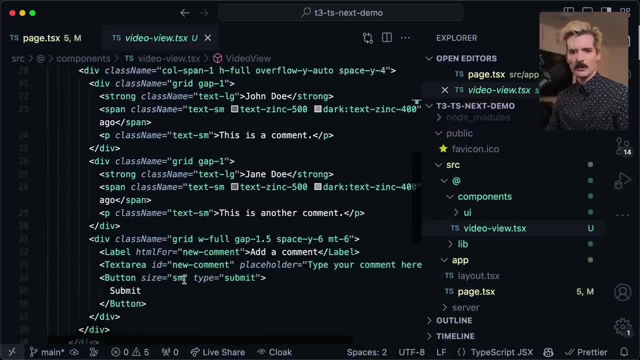 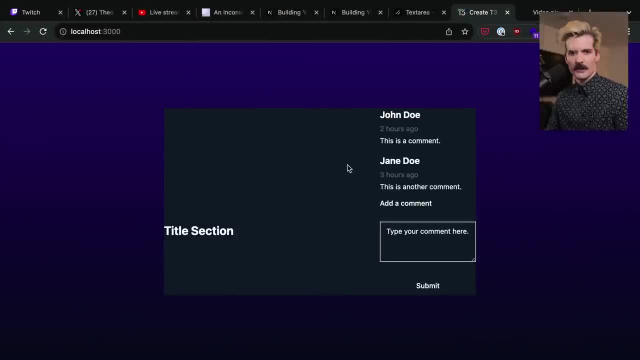 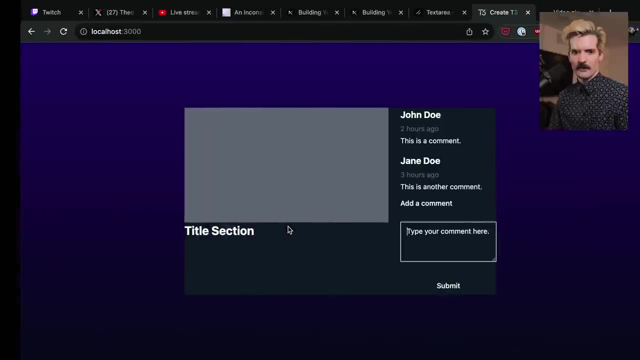 starting point with code and layout and everything else we would need in order to make this look great. I even add a quick background here. just BG gray, Make it darker, And there we go. I wanted to have a background for the video player: BG gray 500.. So 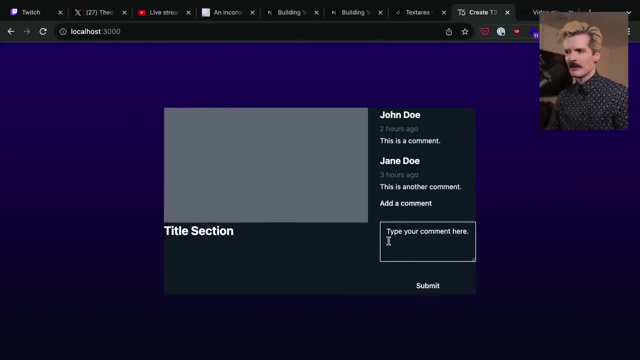 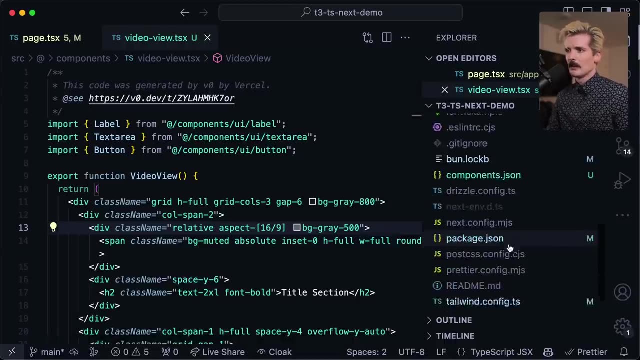 it's clear that like this is where the video would go, And having this in my source code again. this isn't something that just came from the external world in some package that's installed. If we look at my package, JSON, the stuff that's been added is radix is helpers for doing good. 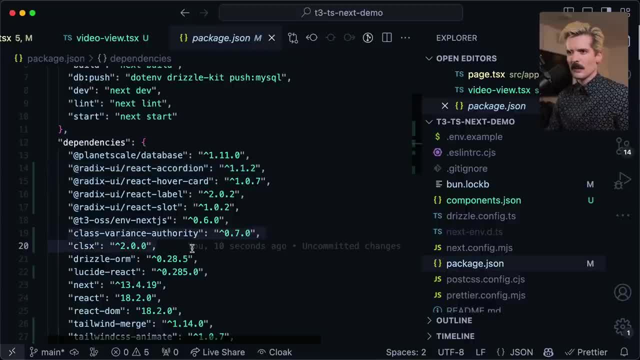 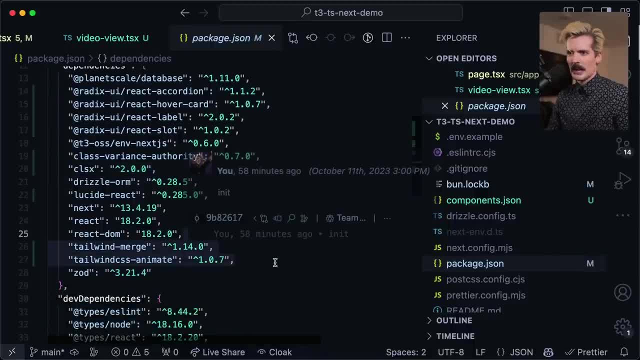 then we have a little bit of code in here, And then we have a little bit of code in here to make sure the right class names are being applied and tail and merge and tail and animate, So you can have your tail and classes merge appropriately and do custom animations on them too. 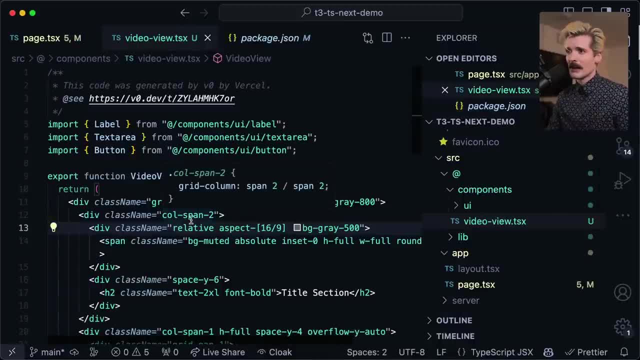 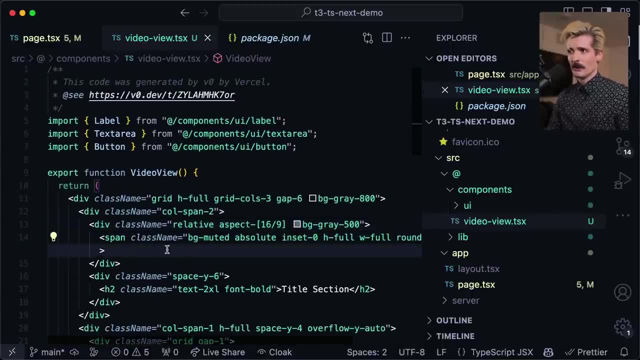 If you've ever built a UI library, your head's probably spinning right now, because this makes all the pieces you need to build a good UI significantly more accessible, and the same way you would have built a package that your company is sharing across things. you can use these pieces. 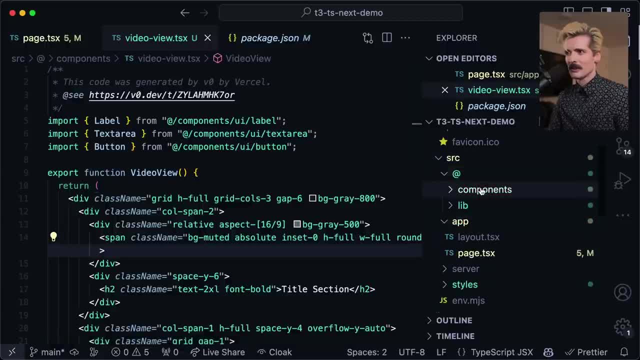 to build that same package, or even just a folder, in your existing application. This has lowered the bar for building a UI library library so low that it's just as good as adopting something like Material UI or like Bootstrap. And since Tailwind is the base piece that assembles all these parts, it's really easy. 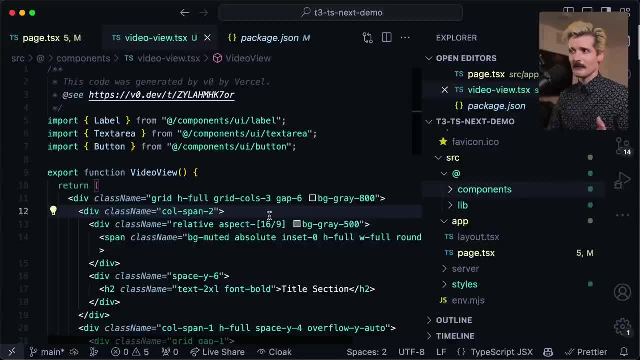 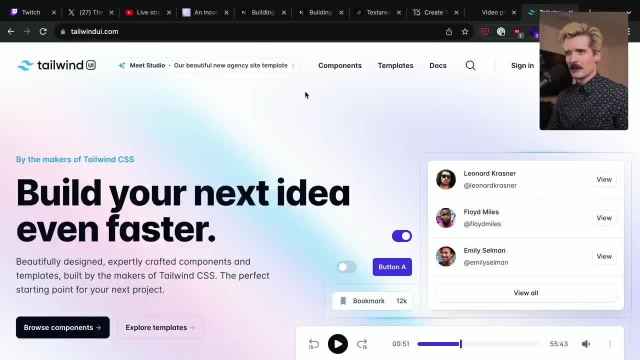 if you've used Tailwind before to make changes to the code that you're getting, be it from v0 or from Shad UI itself. And this isn't the only project that's going in this direction. Tailwind UI is also very similar. Tailwind itself is a CSS library that is just a way to write CSS. 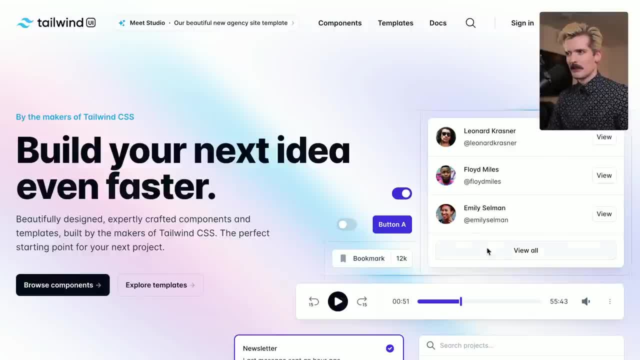 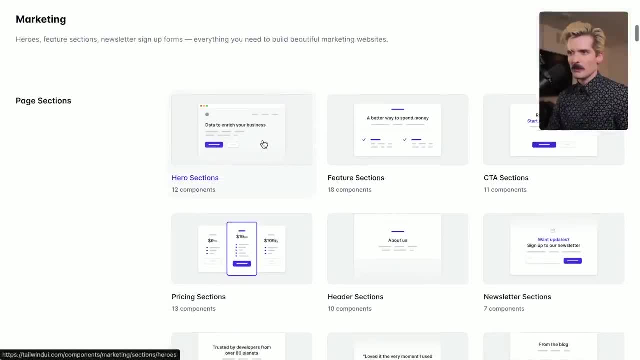 slightly faster. But if you want actual components like buttons, comment sections, audio players and all these types of things, they actually have a bunch of components they've made for you to use And if you want them you go to the page that has the code you want on it. This might look. 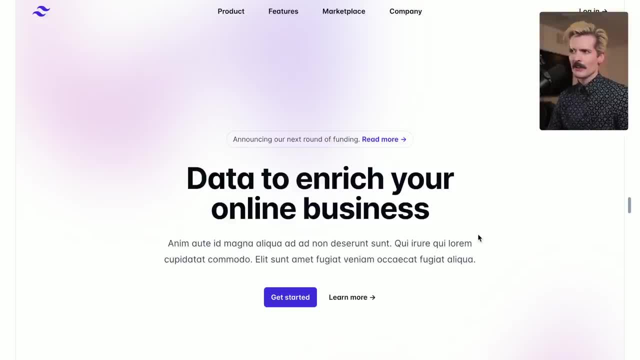 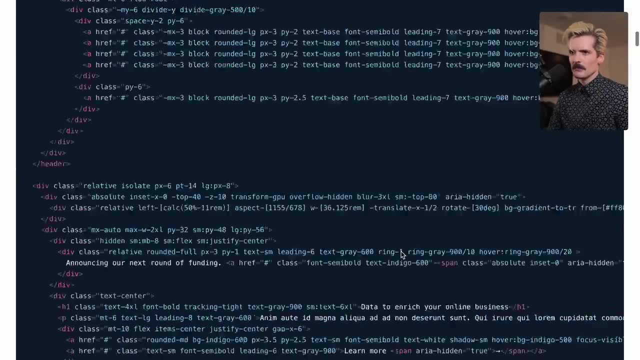 familiar if you've seen the ping or upload things, specifically websites. You can opt to code And here's the source for all of that. Just there for free. free to use you, please. And for the more interactive parts that have, like drop downs and things, they have a little react button too. 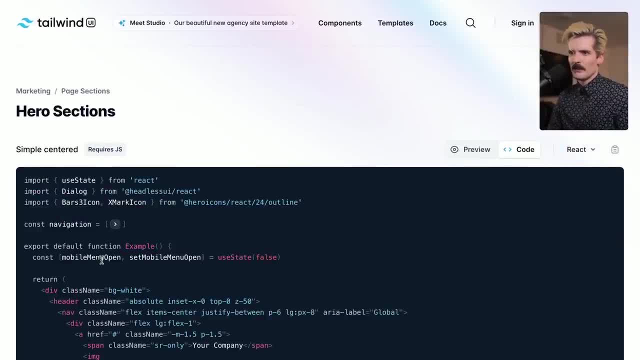 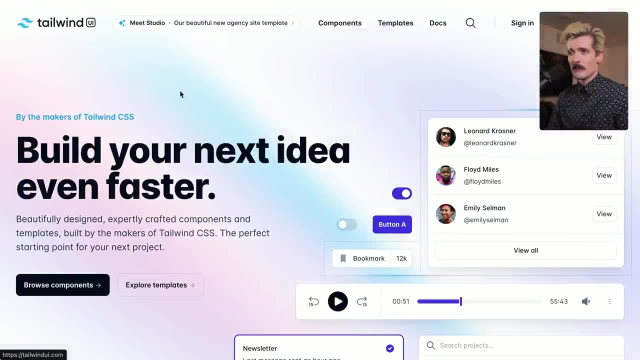 So you can get all the react code. Oh look, it's right there. React, Here's the react code- and even has the mobile menu built for you as well. All of these things are just there for you to use. I will say: Tailwind UI is paid for a lot of it. A handful of the components are free, but they do. 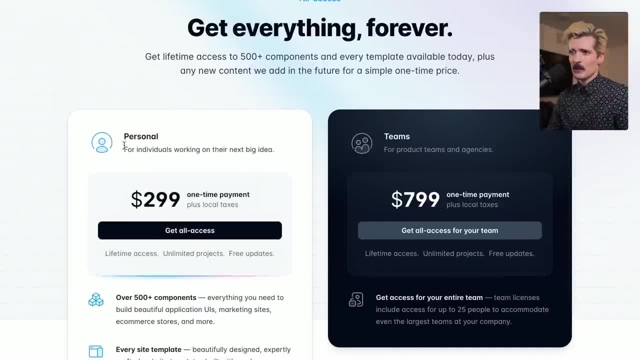 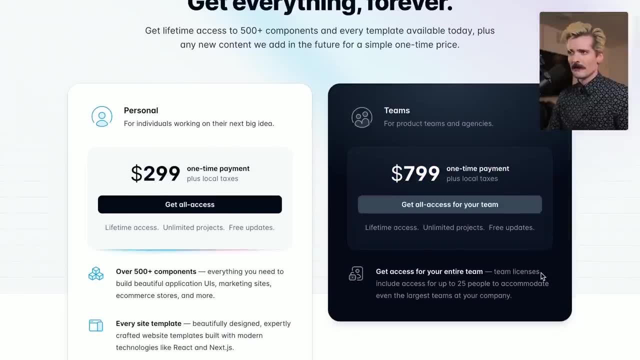 charge if you want everything. It's actually a very reasonable pricing scheme where you pay 300 bucks once ever for just yourself or you pay 800 bucks once ever for your team- Pretty dope. I'm very happy as a Tailwind UI customer and it's really cool seeing things like this especially. 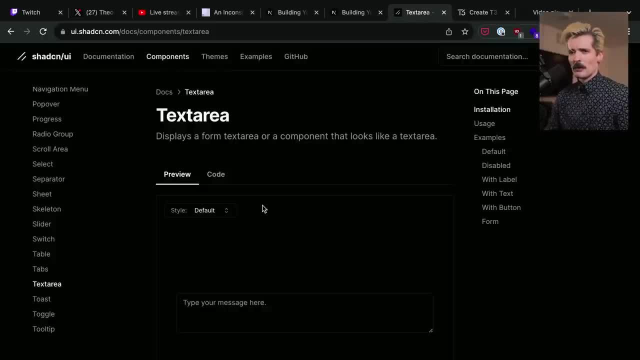 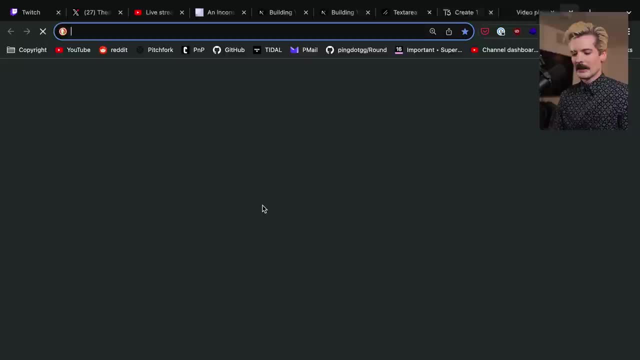 ShadCN and ShadUI Pushing it way further. I wouldn't be doing all of this work justice if I didn't also talk about the underlying pieces that make it possible. Obviously, Tailwind is really big, but I mentioned Radix a bunch. What even is Radix? Radix is a really really powerful set of pieces. 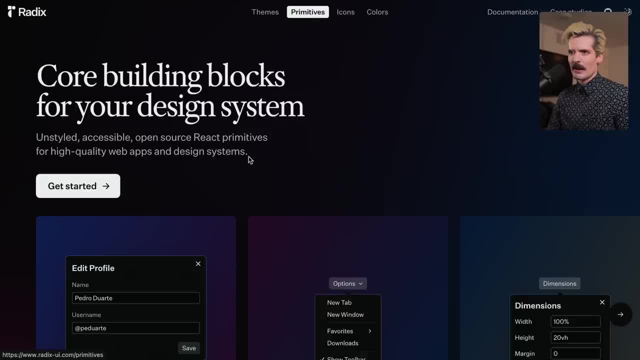 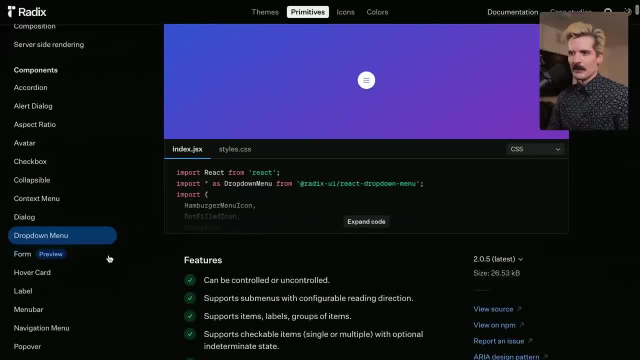 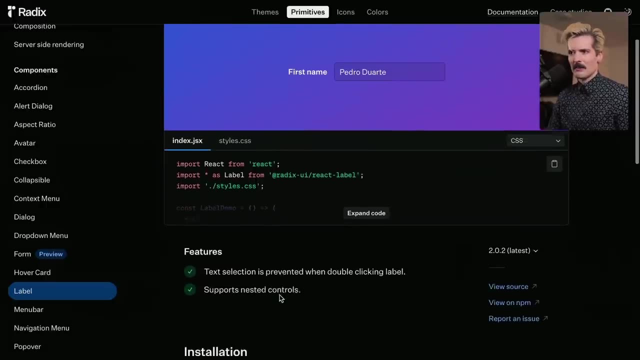 to build accessible react applications. The primitives it provides are incredible. They provide a bunch of hooks and components to do accessible things And this list might look pretty familiar Having a drop down example labels all these types of things. These, these base components and base hooks, are the parts that allow for developers to make really 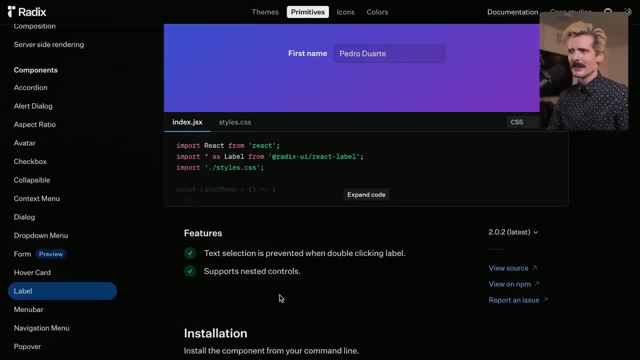 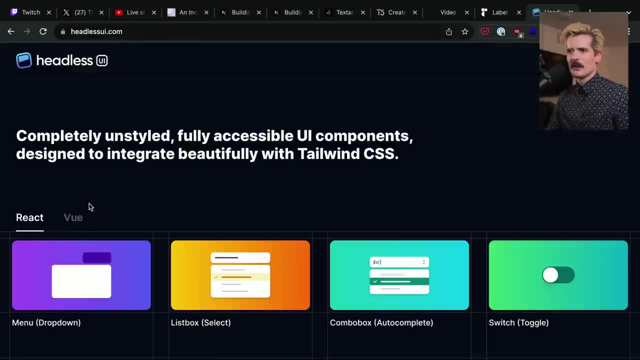 accessible applications and really accessible user interfaces quickly in React and things like it. And it's really cool seeing Radix find success, seeing Headless UI find success. Headless UI is the equivalent of this from the Tailwind team, where they have all of these different components. 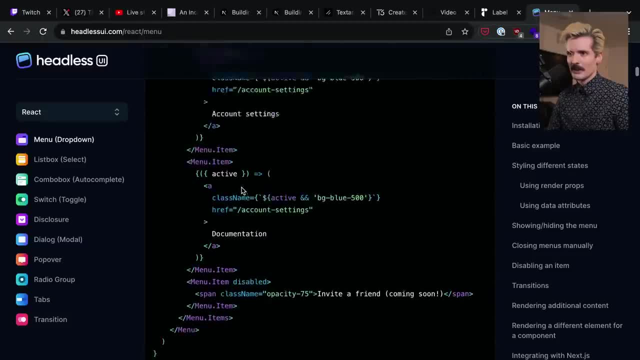 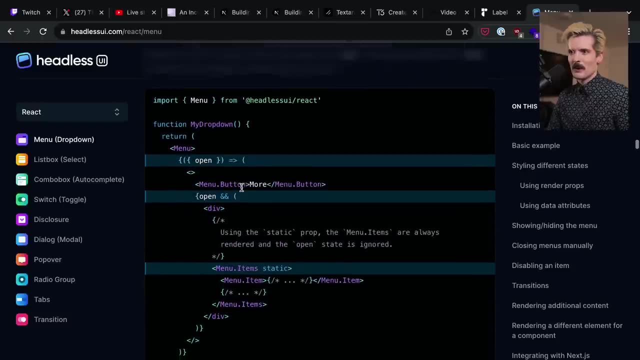 and the hooks and things you would need to run it or render it correctly. It's not just components, it's hooks and behaviors and all of these other complex things that are hard to get just right. And that's why I'm so excited when I see these new solutions, Because getting accessibility, 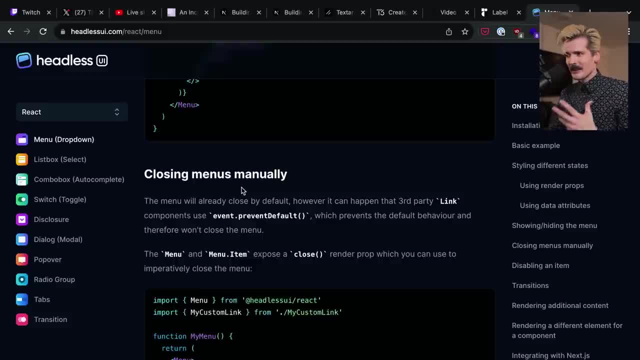 right is hard. Getting your component architecture right is hard. Getting the different states and race conditions and edge cases is obnoxiously difficult And we've been reinventing the same work over and over again. And even if you were using a UI library like a Material UI, 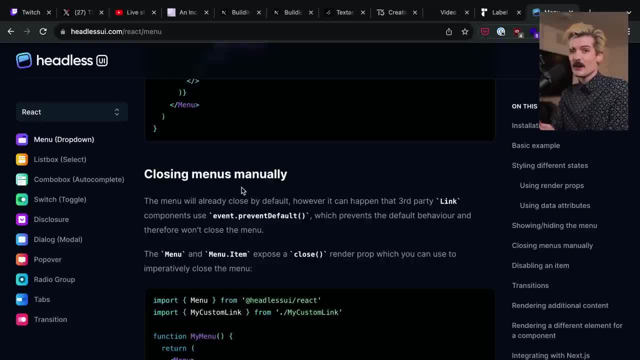 as soon as you had something slightly different from what that provides, it was really hard to build better solutions. on top of it, You end up with a jarring difference between the Material UI components and the custom things you write outside of them, This blurring of the line between library and code you own, where it is always code you own. 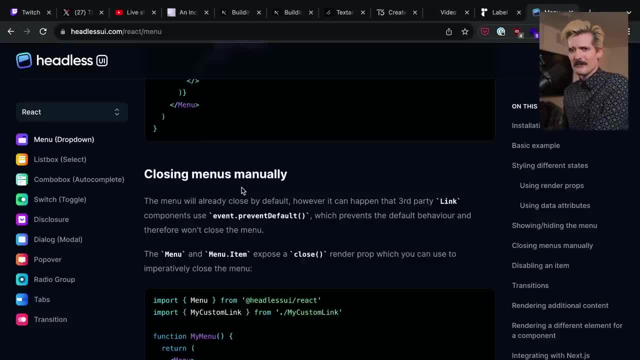 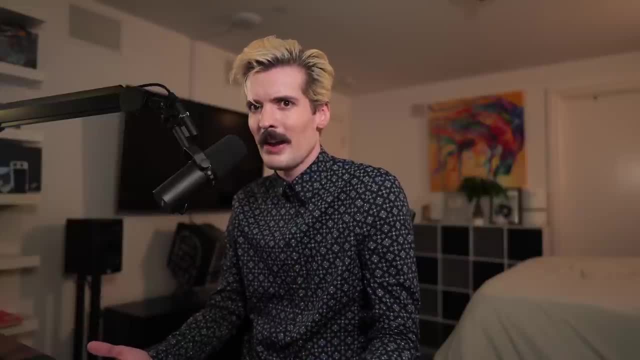 but a lot of the faster movement and agility you normally get from using a component library. you're just in a much better starting point, And that's why I see this transition going as aggressively as it is, And that's why I see so many developers hyped on stuff like Shad UI. 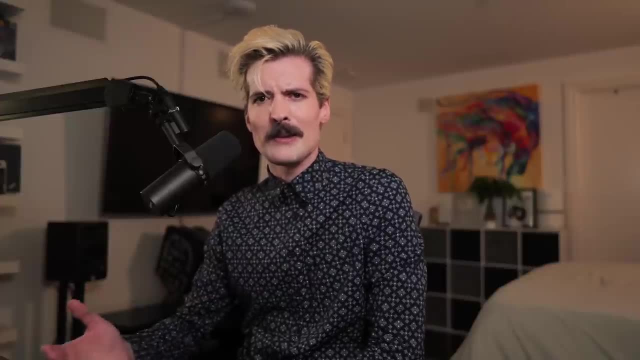 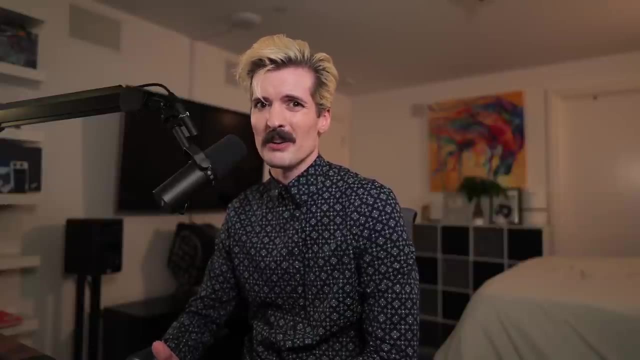 Vercel hired him for a reason. This is very much a bet on the future of how we author applications and user interfaces, And I think I'm making that same bet. I really don't see a future where component libraries are the thing that we're installing in our projects. The future seems.